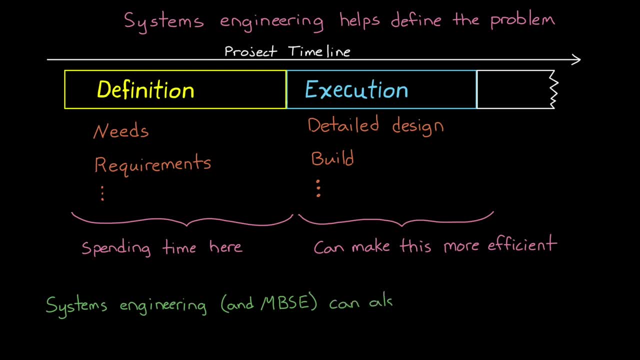 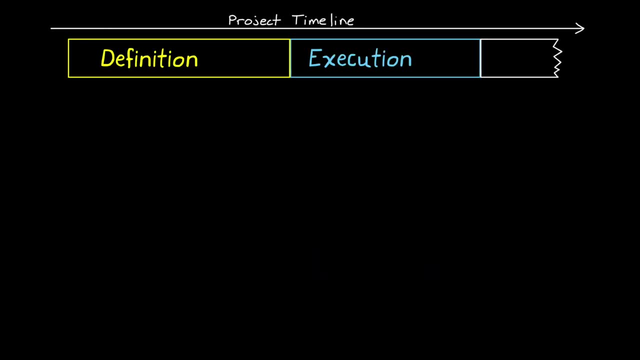 in this video is how much time you need to spend in the definition phase of a model-based systems. engineering can help cut through all of the chaos and get you from definition to execution more seamlessly. I hope you stick around for it. I'm Brian, and welcome to a MATLAB Tech Talk. Let's start by describing this. 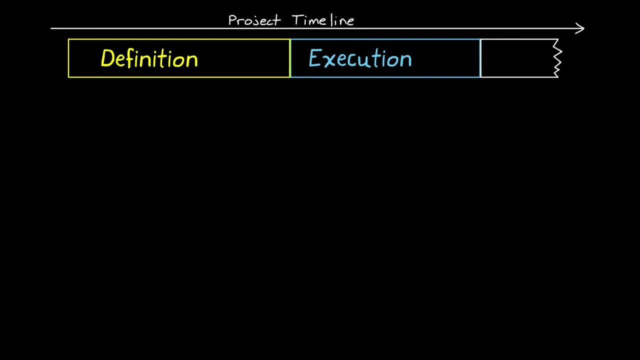 transitional period so that we can understand what drives the chaos. You might be thinking that systems engineering is solely responsible for decomposing the stakeholder needs into perfect descriptions of what the system is, and that the transition from definition to execution is just throwing the requirements and budgets and everything else over a wall to the 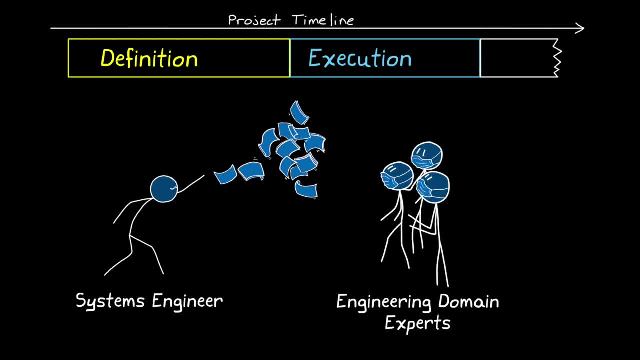 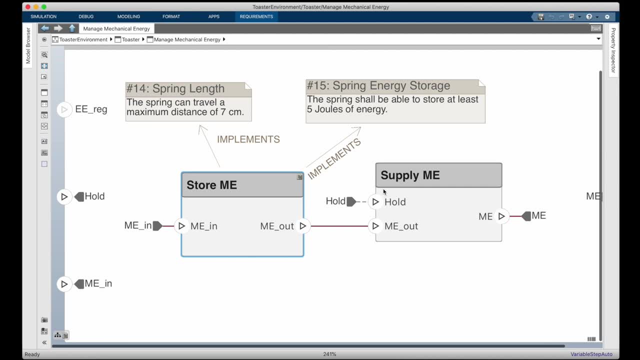 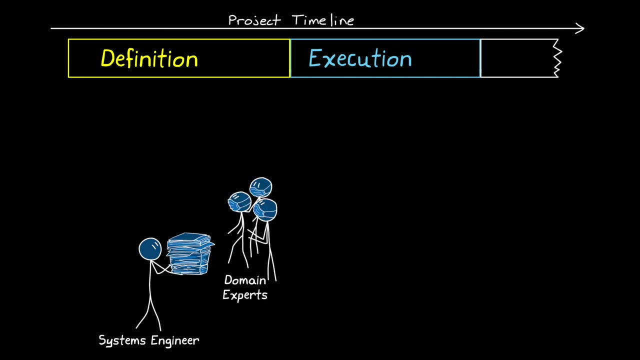 engineering domain experts as some kind of specification that they must follow. This is almost certainly not the case, Remember with the toaster example from the last video requirements. decomposition, which is part of definition, required an assumption about an implementation and this level of complexity can't be done without the domain expert performing trade studies. 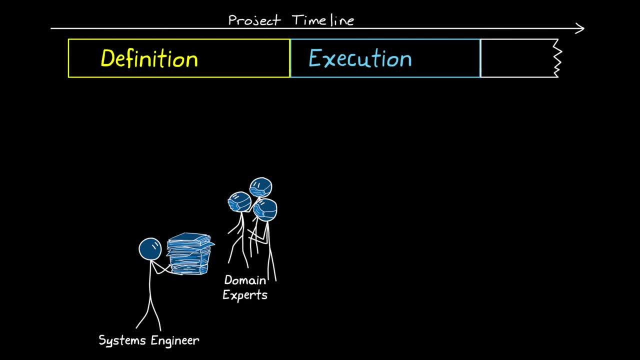 and determining what's feasible and ultimately helping to choose the best implementation to go forward with. and it also can't be done without the stakeholders refining their needs as questions arise and without management to weigh in on the impact to cost, risk and schedule. and so, rather than a one-time handoff, 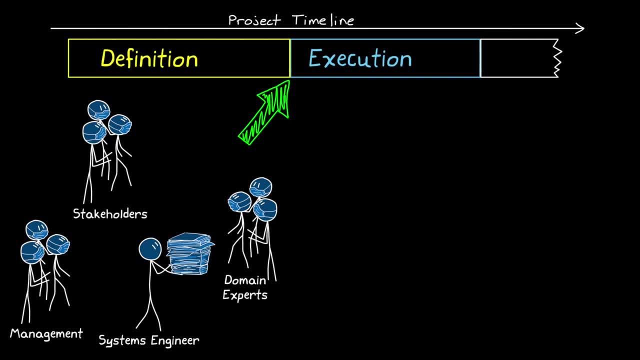 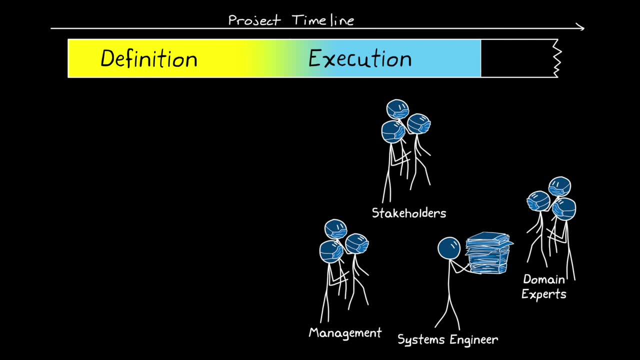 of a completed definition. the transition is more of a fuzzy gradient, as the project and all of the people involved slowly transition from mostly definition into mostly execution. Furthermore, this graphic is kind of giving the impression that the entire project is transitioning at the same time. but complex engineering is messy and often certain. 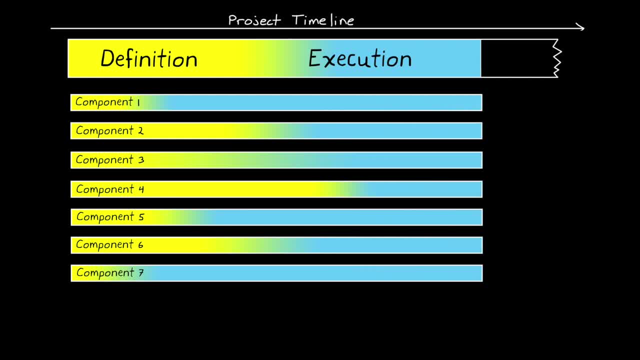 components begin detailed design, while others haven't really been thought about very much, and this might be because some components are naturally simpler and so you can commit to a design earlier. it might be intentionally moved up in the schedule because of a known long lead in procuring some of 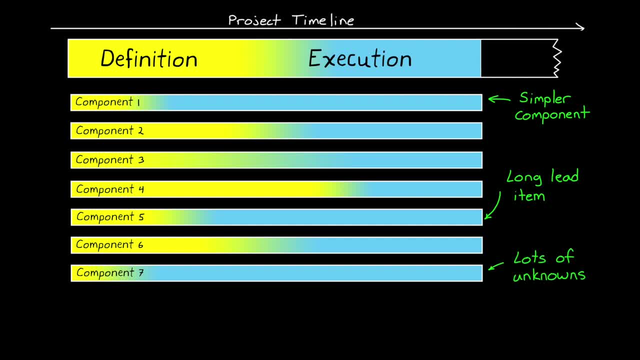 the parts or a component has a lot of unknowns and the feasibility of the entire project is in jeopardy if you don't focus on finding a solution for that component. so you have to start development earlier. but regardless of the reason, this simple gradient is really many different gradients that. 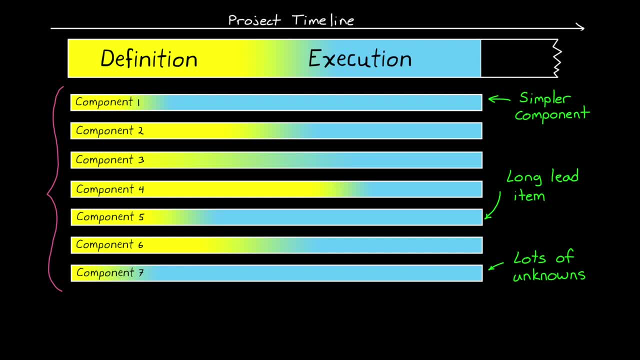 represent the transitions of each of the major components or sections of the system. and to complicate this even more, this isn't always a one-way Street, where you define the features of a component first before doing a detailed design and building it. sometimes you start with one or 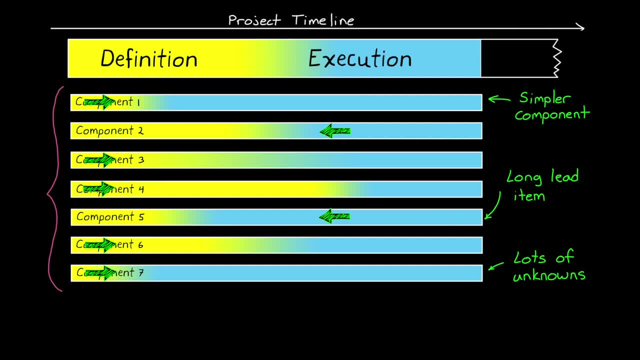 more existing components and you have to figure out how to fit them into the definition. for example, you might be reusing software or hardware from a previous project. this is common in the automotive industry, where the same engine or transmission or some other part is used across multiple models. in this case, the component is fully developed and you have to define the rest. 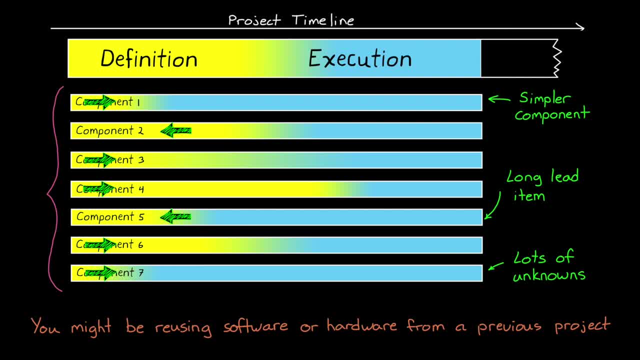 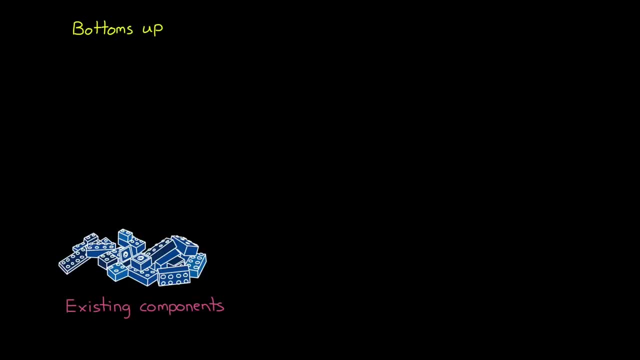 of the system so that it works with it. now a real quick aside: if you are building a system completely by reusing existing parts and you don't have a sense of what you want the final system to do, this is a bottoms-up approach to engineering. it would be like starting with a 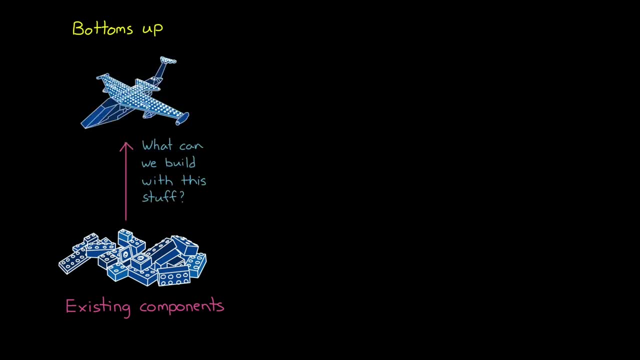 collection of Legos and then snapping them together to see what you can create. you don't have a grand idea of the end product. you just see what emerges from the available parts. the top-down approach, on the other hand, would be starting with an idea of what you want to create and then figure out which. 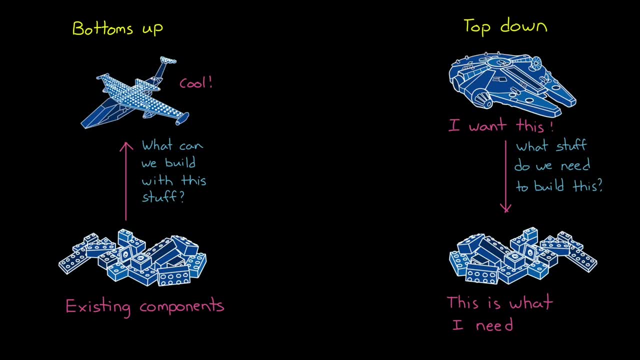 parts you need in order to accomplish it. however, more often than not, we're doing some sort of meat in the middle approach, where some of the components might be fully fleshed out and designed already and you have to incorporate them along with other components that aren't built yet in a way that 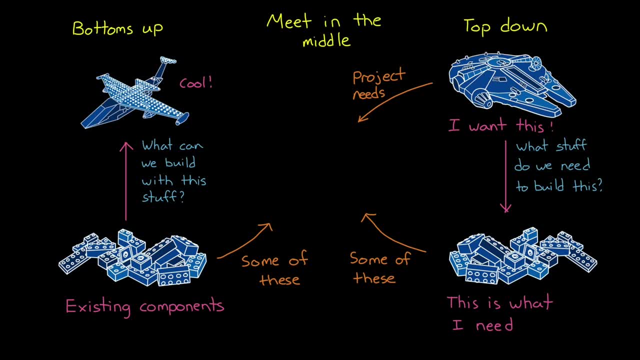 meets the overall project needs, and so in the definition phase you have to make sure that the design you're coming up with has compatible interfaces with these existing components, and that the items that flow into the component exist in your system and that the requirements for that component are incorporated. 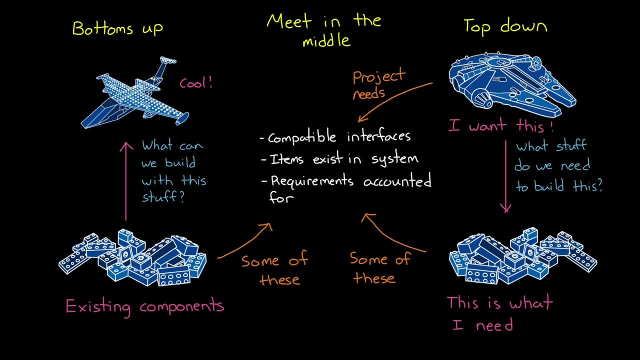 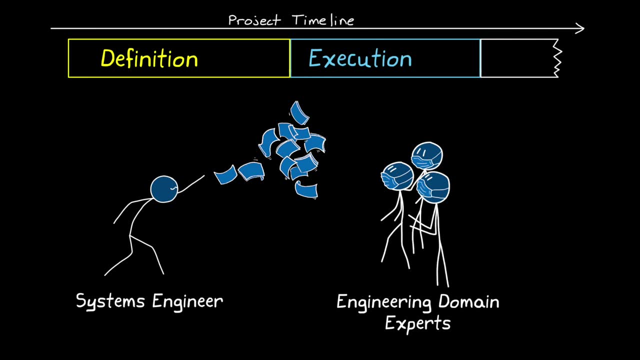 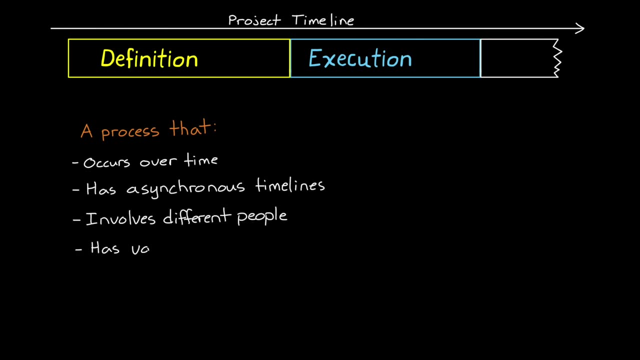 into the requirement hierarchy. all right back to this transition. hopefully you can see how this is much more complicated than a one-time handoff of the definition. it's a process that occurs over time with asynchronous component timelines, and involves different groups of people and has components of varying levels of. 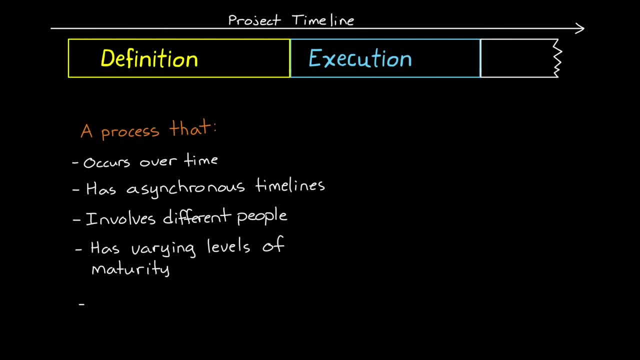 maturity. it's a transition where people are still decomposing the system into functions and components and writing requirements, while simultaneously trying to perform trade studies and make design choices, and the goal of systems engineering through all of this is to make sure that all of the people and components and system design stay compatible and consistent with each. 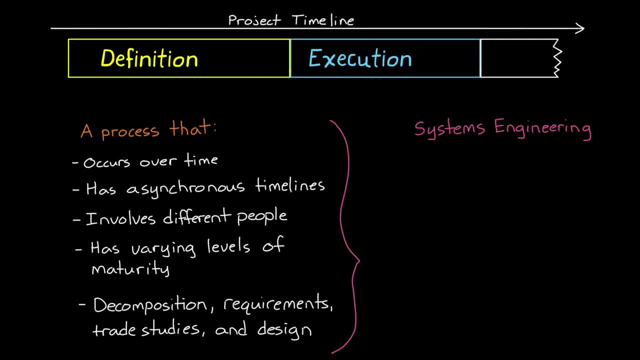 other, and that they're still continuing to meet the requirements of the system and that they're continuing to meet the needs of the project as a whole through this entire transition- and this is where model-based systems engineering can Shine. models are valuable because we can execute them. 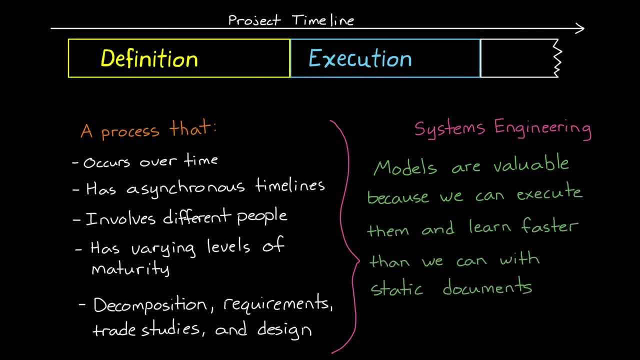 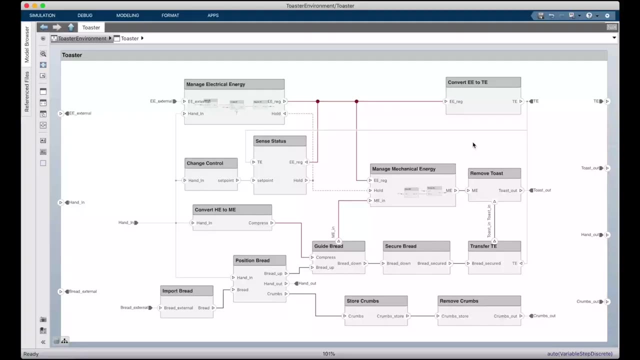 and learn something about the system faster than we could. with static documents that have to be updated and interpreted manually, and in the early chaotic stage of a project, fast and accurate information for decision making can make a huge difference. we can kind of get sense of the benefits of models by expanding on the simple toaster example from earlier in the 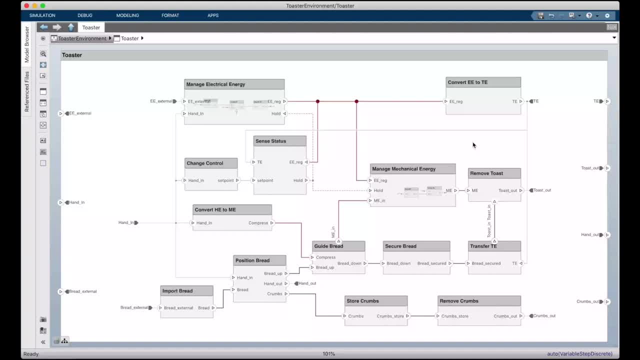 series A systems engineering team working with management and the stakeholders, have decomposed the high-level program needs into an executable functional architecture. But in order to decompose, say, the heating function further and to write lower level requirements for it, the domain experts need to get involved and start trading possible implementations With a model like this. 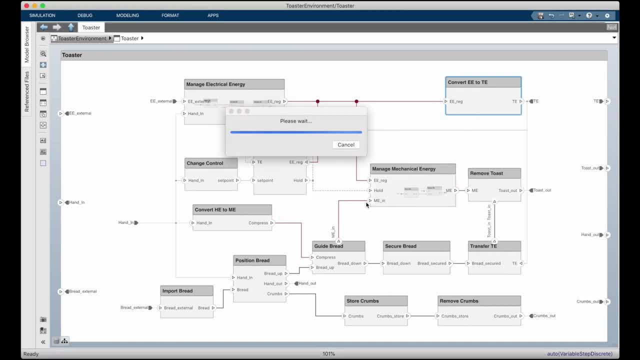 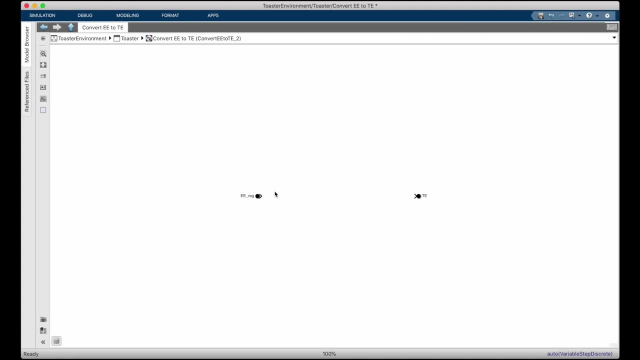 they can start from the function definition itself. In this way, the domain experts are given something to start from which would ensure that things like the interface to that function is consistent with what's needed at the system level, And then, starting from this, they can model. 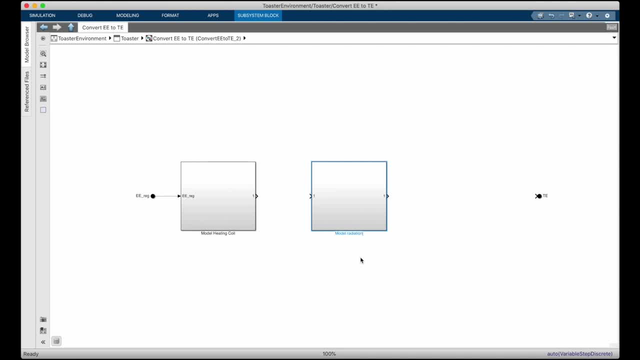 the physics of different implementations that they believe can meet the heating needs. So in this way the model provided the definition of the interface, the requirements and the requirements of the interface, And then they can start from the function definition itself, All of the things that go into the definition in a convenient way. But it also provided the 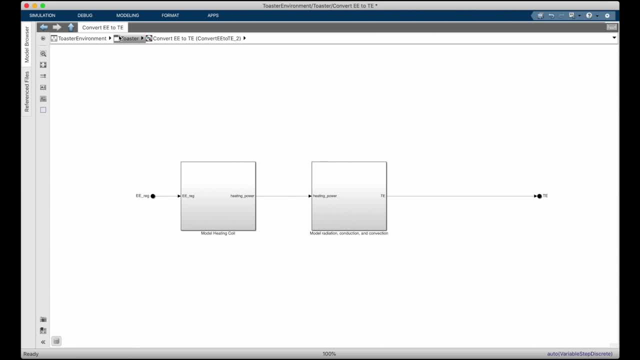 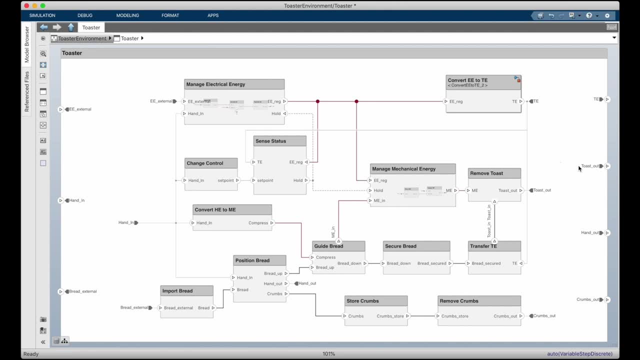 structure around which the domain expert could complete their design. But that's just one component. At the same time, other components are undergoing similar trades and each of them are at different levels of maturity as they progress from mostly definition to mostly execution, at their own rate. Of course, if we are reusing components, and those components already have models created, 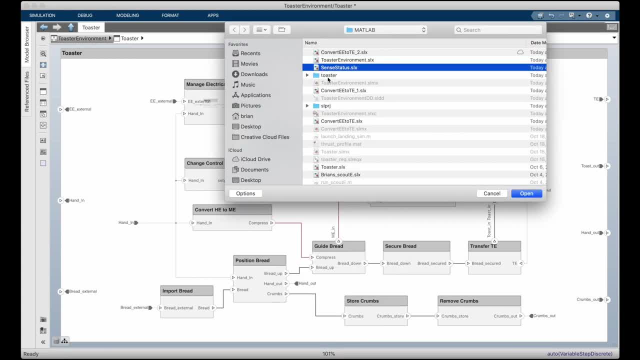 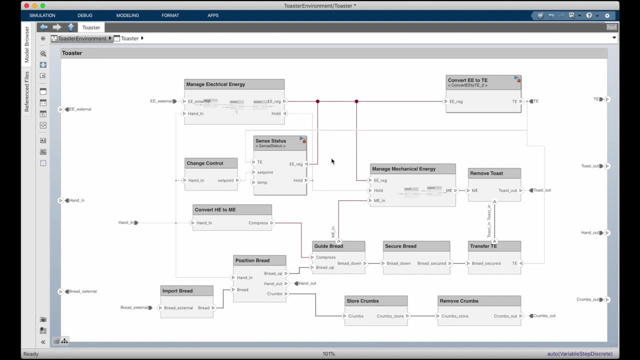 we just pull those models in as is And through this whole process we monitor for interface violations or constraint violations or any other mismatches in the design, And if there are any violations we can catch that before we go any further into the design and then make changes. 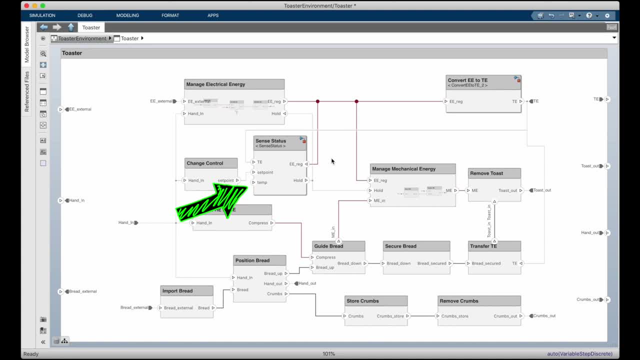 to the components or implementation to address it. Now, in addition to this sort of checking violations, as component models are created, we can also simulate the system level model To verify performance measures are being met. So model based systems engineering and model based design can work together to provide a testing framework that can be used for the individual. 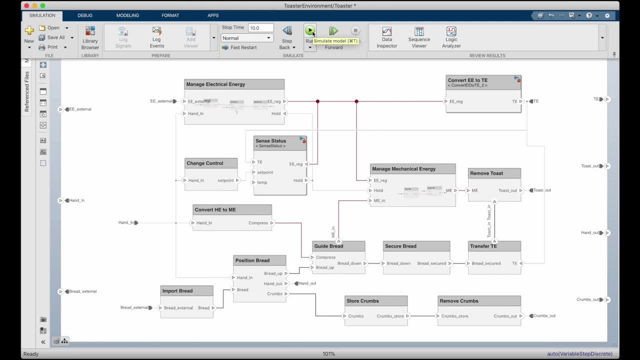 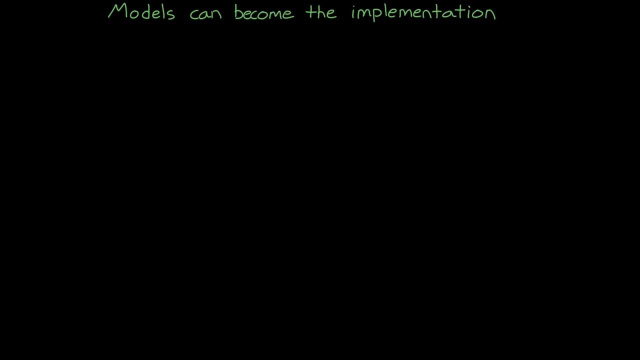 components and for the full system verification. And one more thing that I quickly want to mention here is that the models that we build as part of defining the system, especially for software based systems, These models can become the actual implementation. So a model can be more than just a definition or a starting point for the implementation. 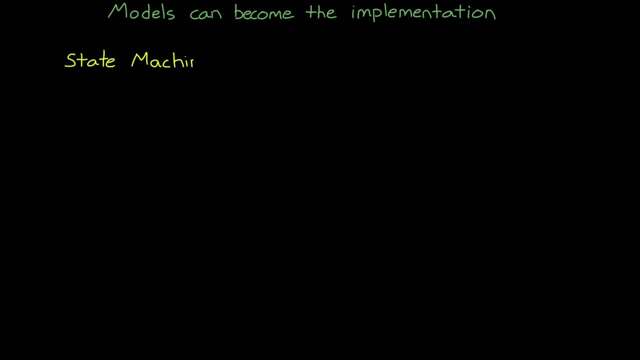 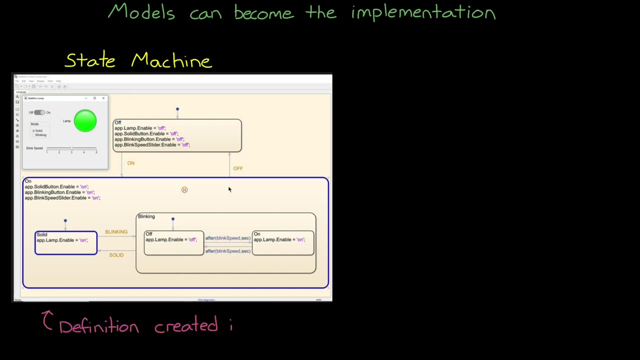 They can be the implementation. For example, a state machine defines the different states of a system and how the system transitions between those states. The definition is built into this representation And someone could write the code for this state machine as it's defined. But we can also generate: 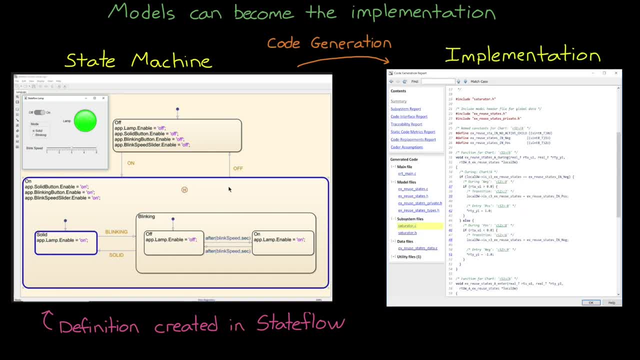 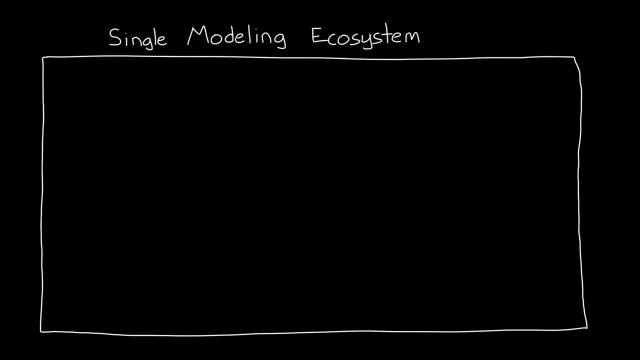 the production code for the state logic directly from the model. So the human readable diagram that defines the states and their transitions is the source for the code itself. Now there's this dream in model based engineering where a single modeling ecosystem could capture the stakeholder needs and then requirements definition and